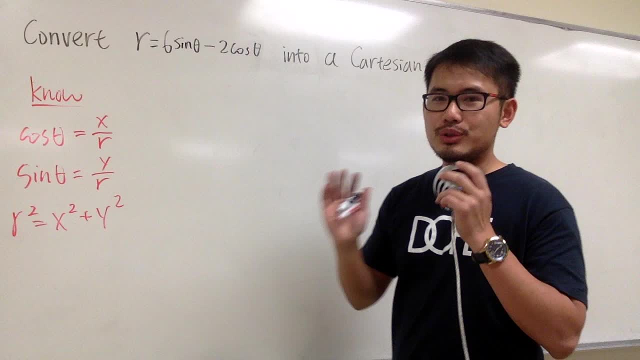 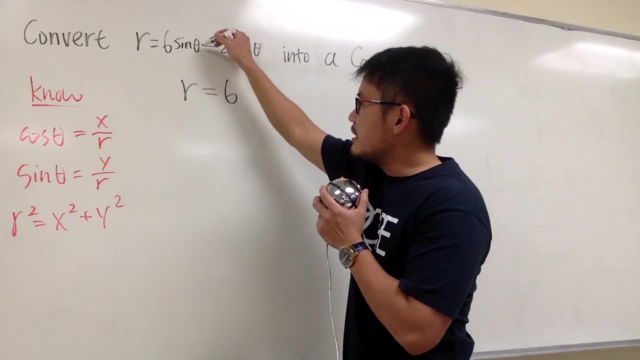 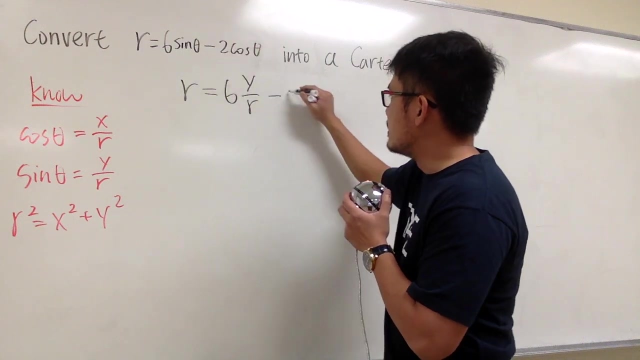 and we can plug in these two things into here and here. Let's do that first. So we have r equals to the 6 states the same. but then for sine theta I will put in y over r And then we minus the two states the same. cosine theta is x over r. 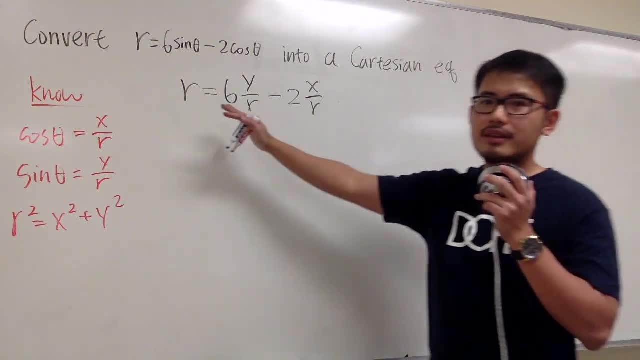 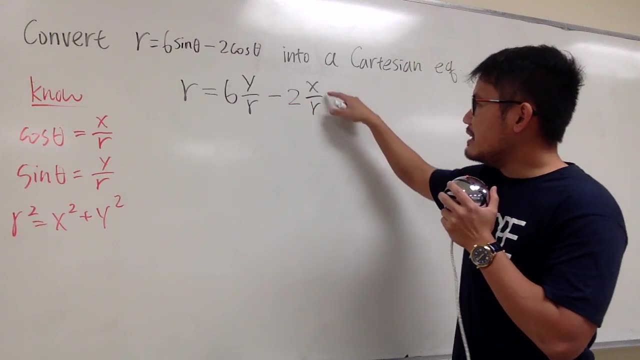 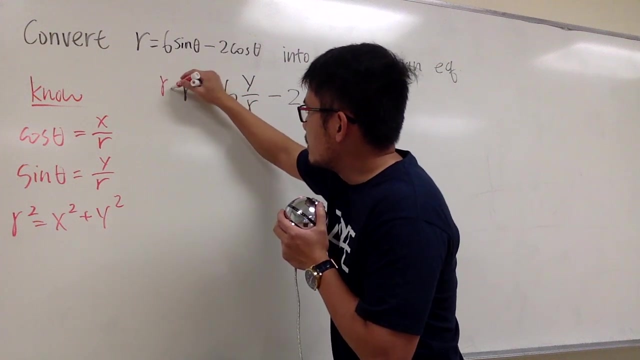 Okay, so this is the first thing that we should do. And then you see that this is the equation that has fractions. We have y over r and then x over r. How about let's multiply everything by r? together, We'll get rid of the fraction. So let's do that. Multiply this by r. multiply this by r. 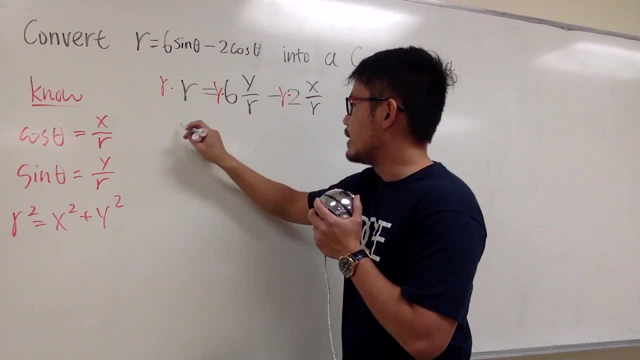 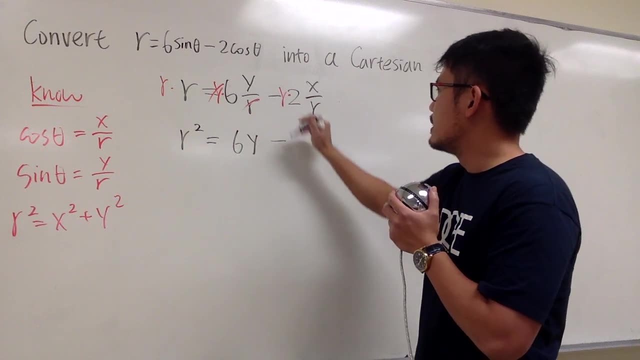 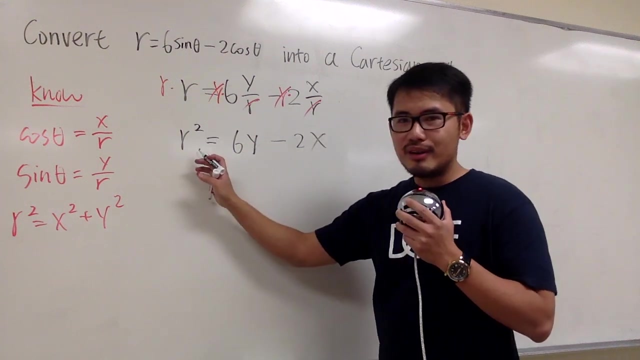 and then multiply this by r, So you see that we get r squared equals to this r and that r cancel 6y minus this r and that r cancel minus the 2x, like this, And then what's r squared? We know r squared is the same as x squared plus y squared, So I can plug this in here. 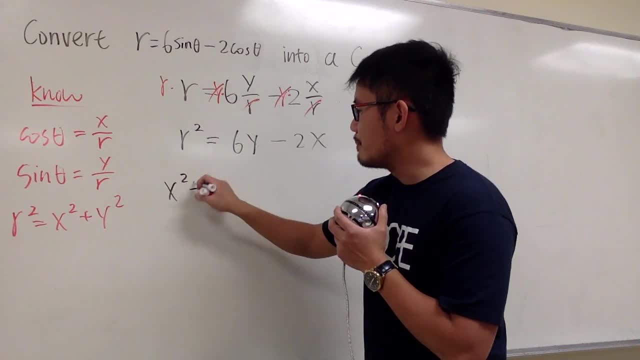 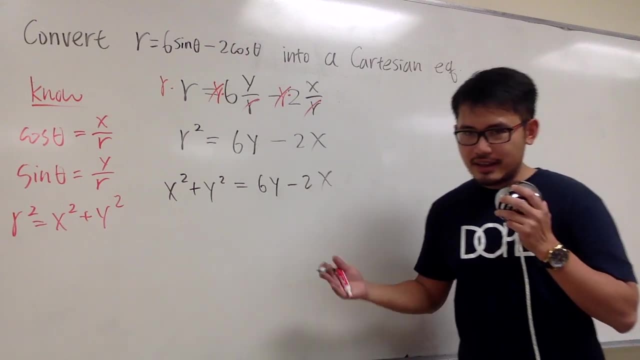 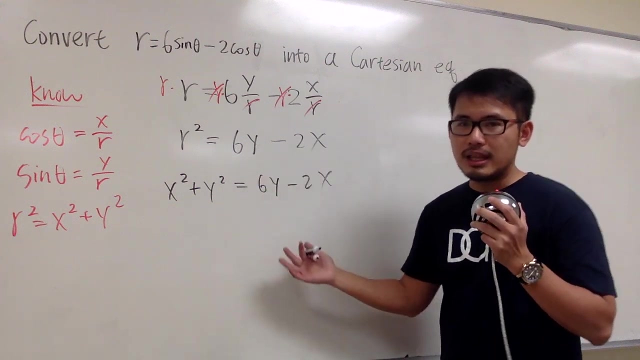 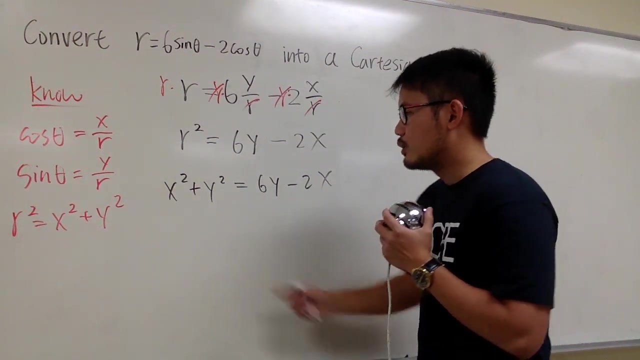 this is going to be: x squared plus y squared equals to 6y minus 2x, And technically we are done. but we can do better, because I cannot really describe how does this equation look like in the Cartesian equation world. right, And this is how we continue. Let's move this and that to the left-hand side, So let's add a 2x. 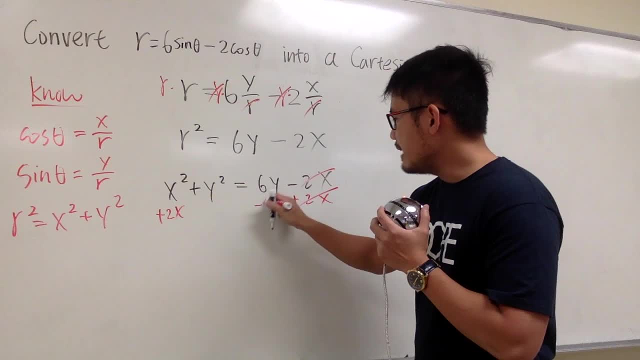 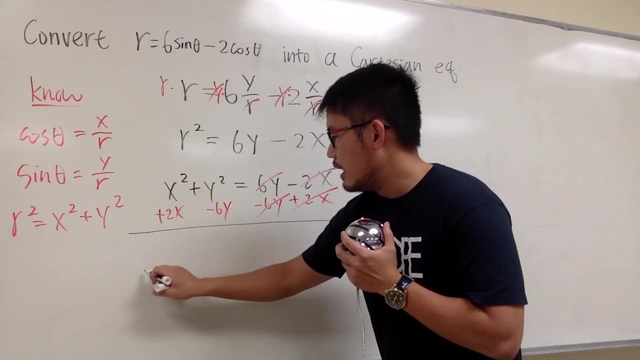 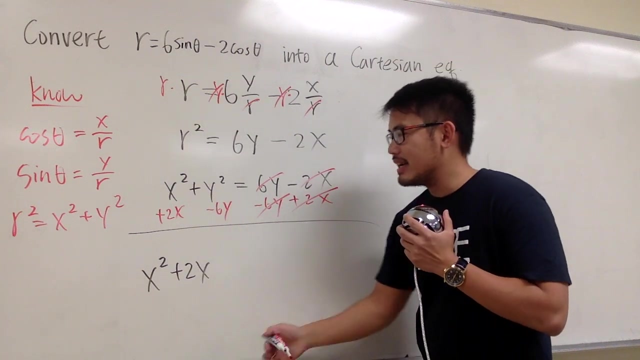 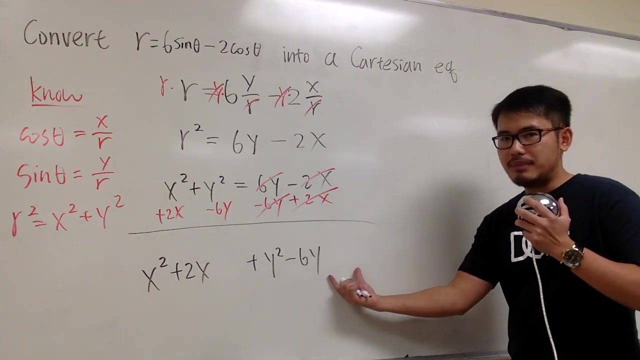 on both sides And that's minus the 6y on both sides. okay, Altogether, we see that we have x squared plus 2x, And then let's leave a space. Continue by putting down plus y squared minus 6y and leave a space equals to 0.. And why do I have 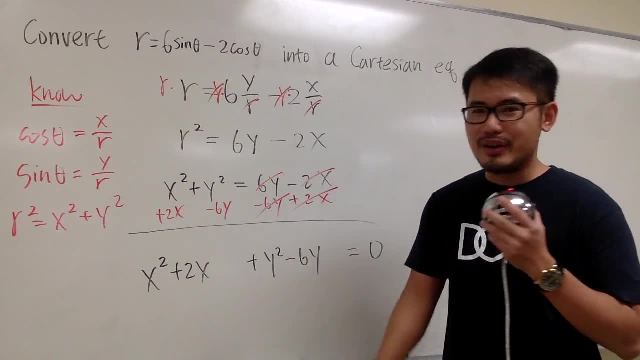 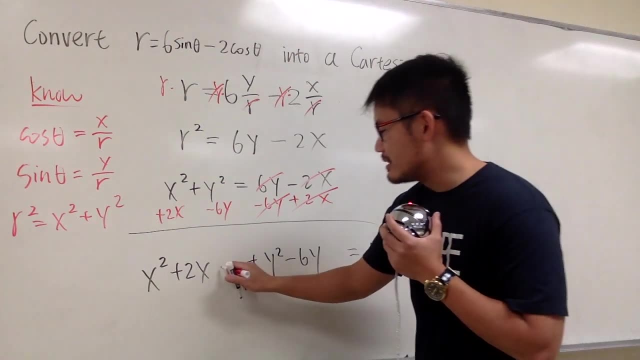 to leave a space Because I want to complete the square. This is x squared plus 2x. Let's add a magical number. That magical number is plus 1.. How do I get a plus 1?? Well, to work this out.